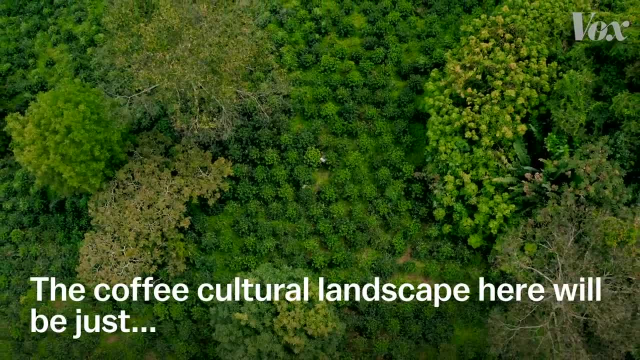 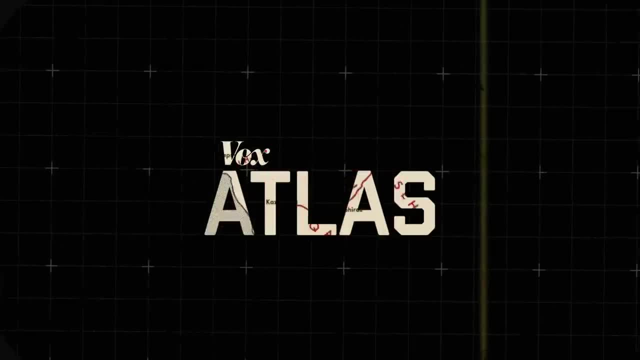 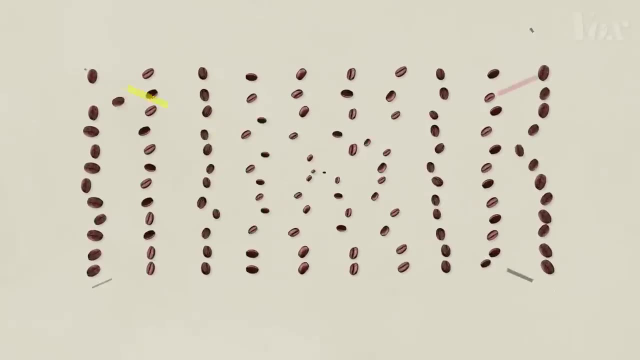 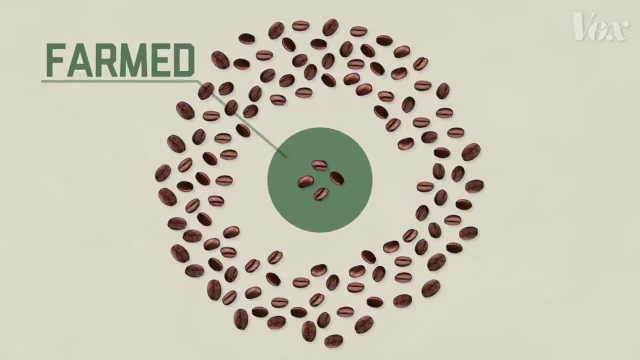 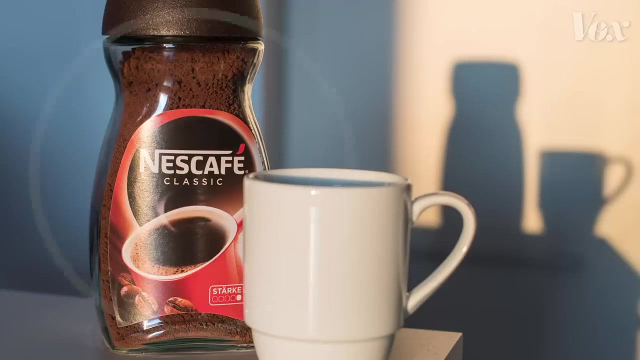 that coffee culture will be a memory. There are over a hundred species of coffee plant. The vast majority occur in the wild, while a few are cultivated on a farm, Two of which are by far the most common. Robusta coffee has a bitter taste and is used to make espresso and most instant coffee. 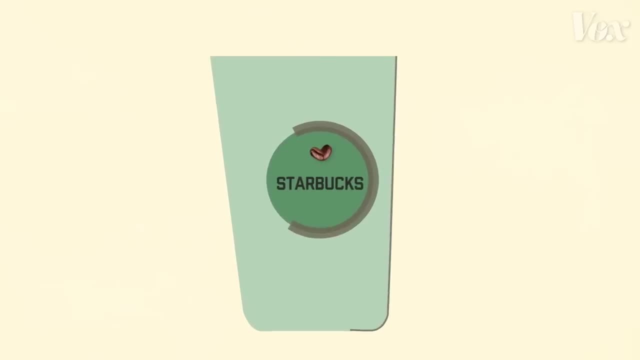 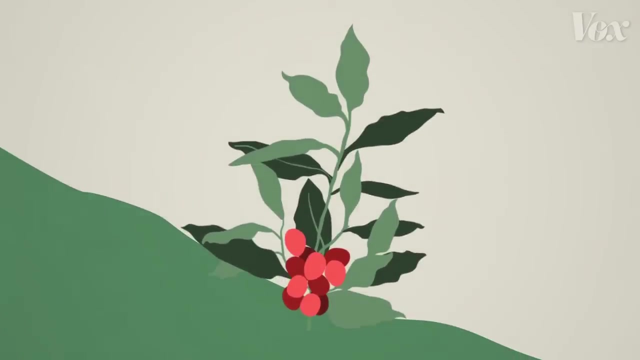 Arabica coffee is the good stuff. It has a smooth and mild taste and is used for high-quality coffee. Both species require specific conditions to grow, but Arabica is particularly sensitive. The plant needs temperatures between 18 and 21 degrees Celsius. 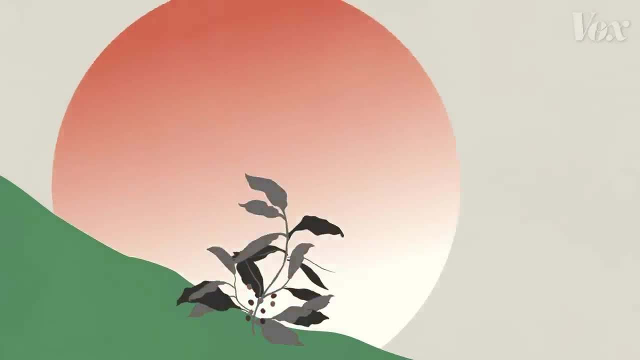 Too hot and the berries won't grow correctly. Too cold and it can freeze. It also needs a specific amount of rain, preferably with a three-month dry season, to flower And, crucially, it needs warm days and cool nights. so it grows best at a certain elevation. Altogether, that means Arabica grows best between these latitudes, And if you were to create a perfect place for it, it would look a lot like Colombia, Specifically the Zona Cafetera, Colombia's coffee region. We have a wide variety of climates. 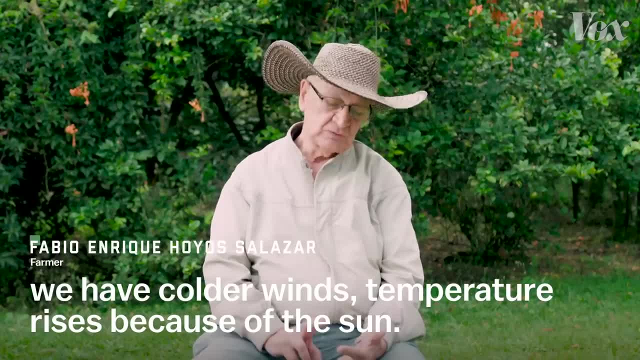 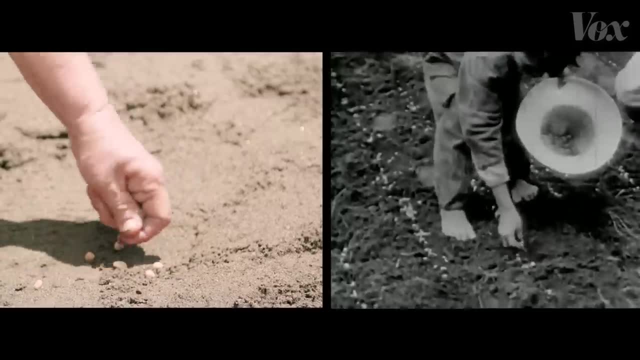 We have waters, we have colds, we have heat from the sun. The coffee farmers grow and process it all by hand here, which is why Colombian coffee has been considered the best in the world for over a century. We love it because we were born with it. 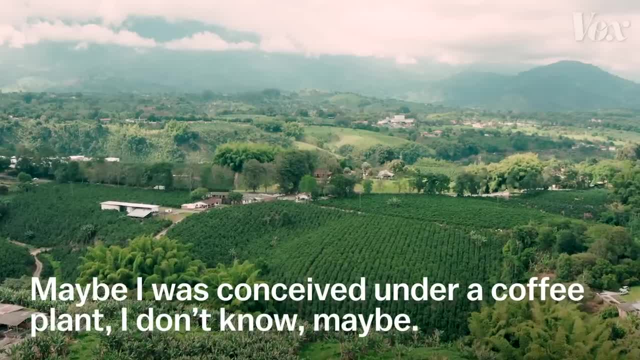 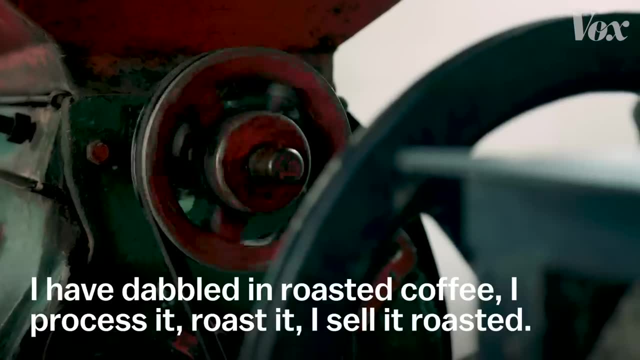 That's how we were raised. Maybe they told me it was under a coffee stick. I don't know. Maybe I'm very fond of coffee. I've been into toasted coffee. I process it, I grind it. When it's toasted it's an art. 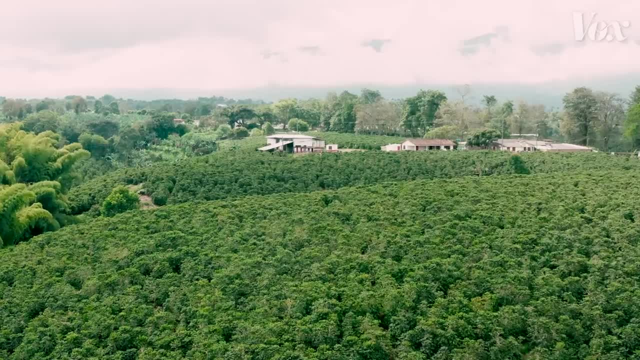 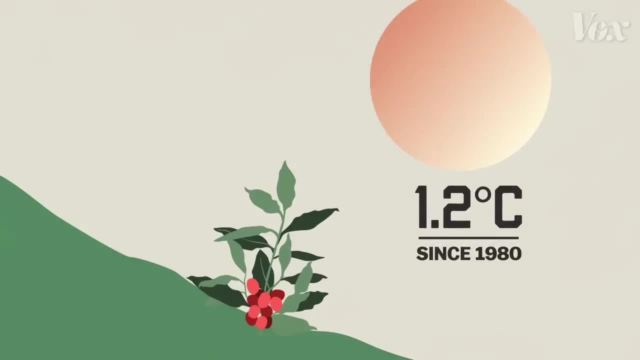 It's become an art. But the Zona Cafetera is also where climate change is already taking a toll. Greenhouse gas emissions have warmed the region by 1.2 degrees Celsius since 1980. That's enough to push the optimal elevation for coffee higher up the mountain. 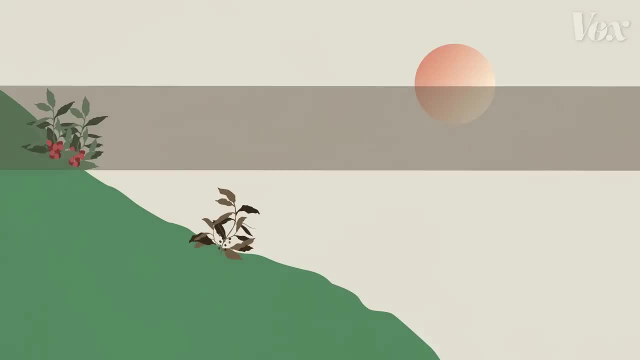 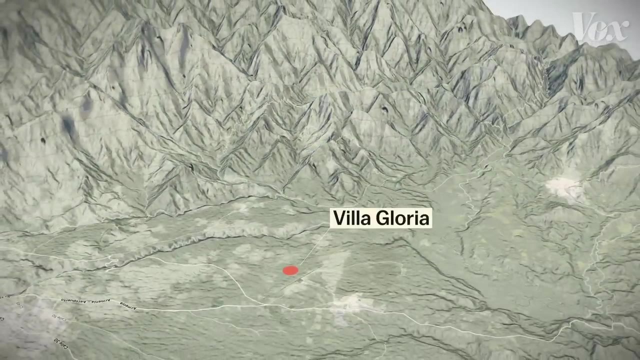 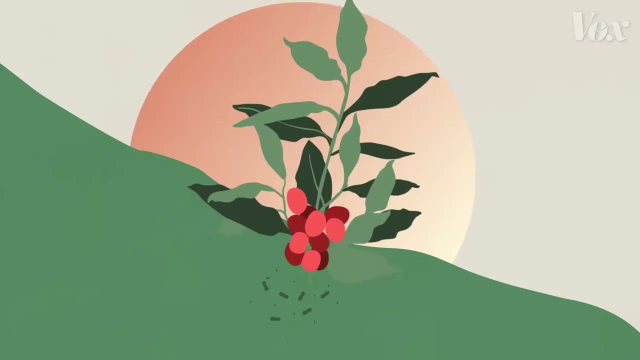 leaving the plants down here to overheat and produce lower quality beans. That's what's happened here. on the Villa Gloria farm, which sits at a low elevation, We've had unbearable temperatures and sunsets that didn't exist in years. The warmer climate is also ideal for pests and fungi. 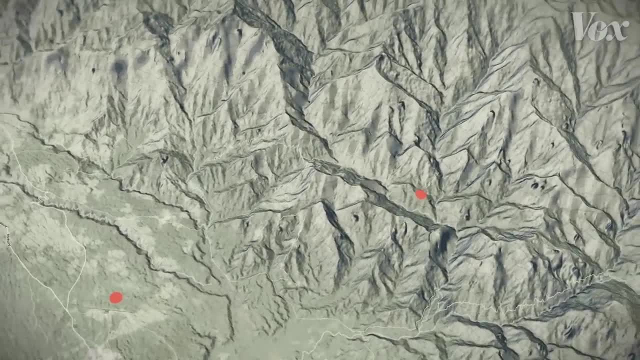 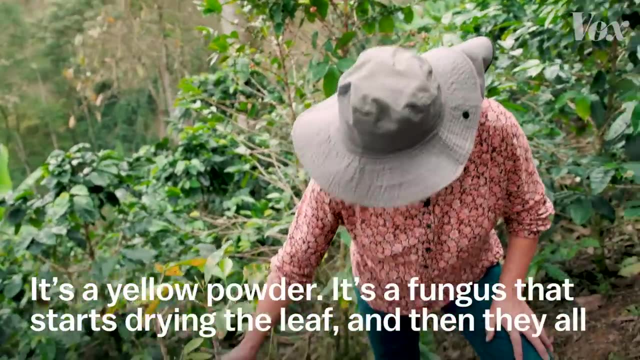 Up the slope. some coffee plants at the Santa Fe farm are afflicted with a fungus called coffee rust. It's a yellow powder. It's a little fungus that dries the leaves and they all fall. As you can see, there are no branches here. there's nothing. 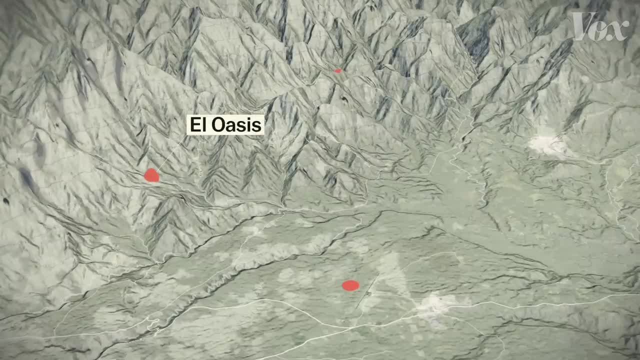 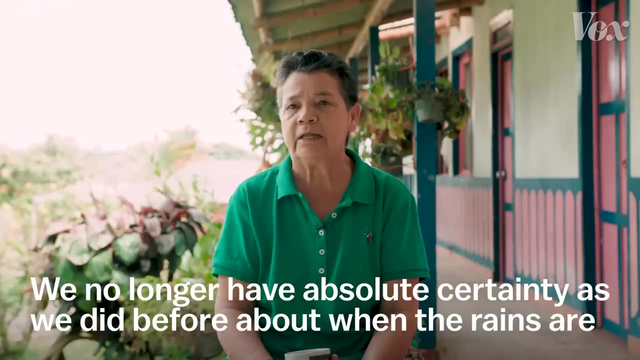 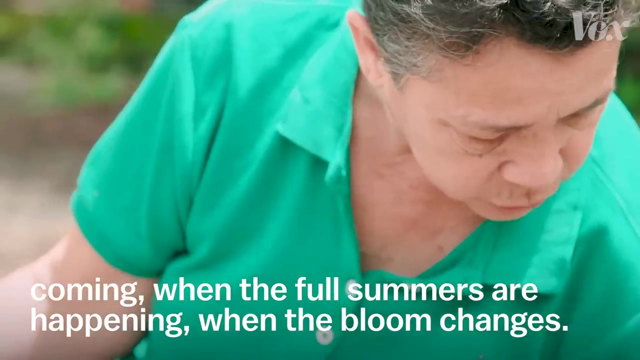 And here at the El Oasis farm. changing weather patterns have made it hard to predict the life cycle of coffee. So it has changed, that we no longer recognize with absolute certainty when it rains, when it's full summer, when it's flowering. We have to be aware that the flowering has changed. 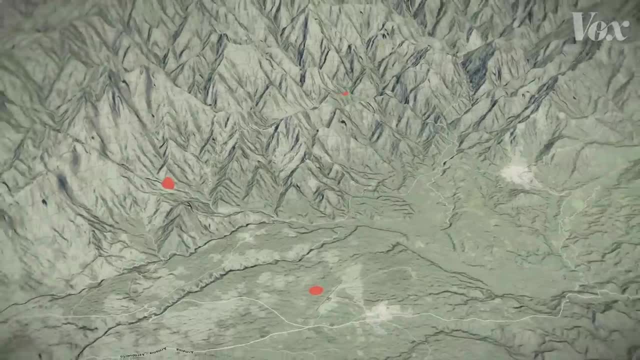 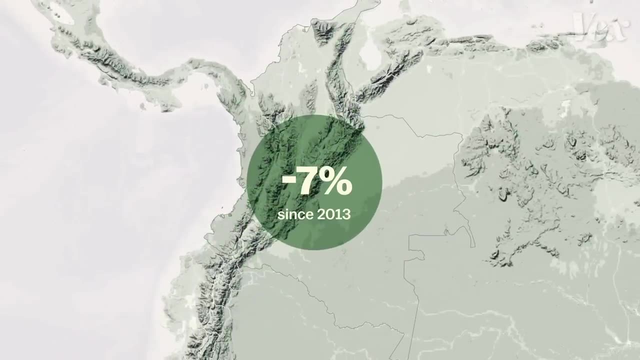 And that's thanks to climate change. Since 2013,, the amount of land used to grow coffee in Colombia has fallen by more than 7 percent, And scientists expect things to get worse. The Zona Cafetera is projected to warm by 0.3 percent. 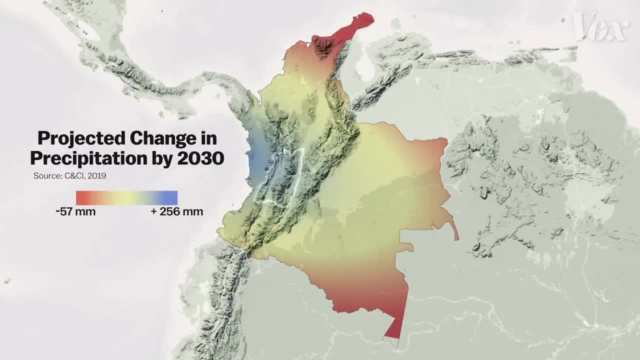 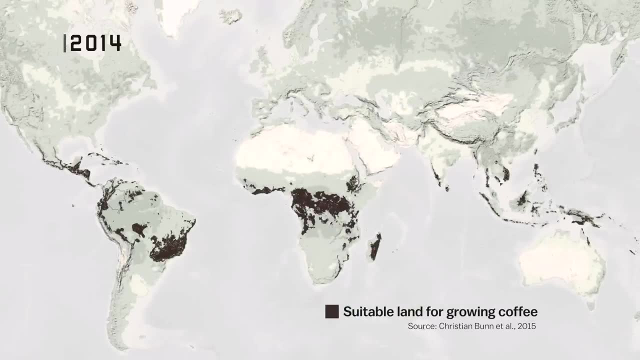 at 3 degrees per decade and see more extreme weather. In fact, coffee-growing regions everywhere are going to be affected. A recent study estimates that by 2050, the amount of land that can sustain coffee cultivation will be reduced by 50 percent. 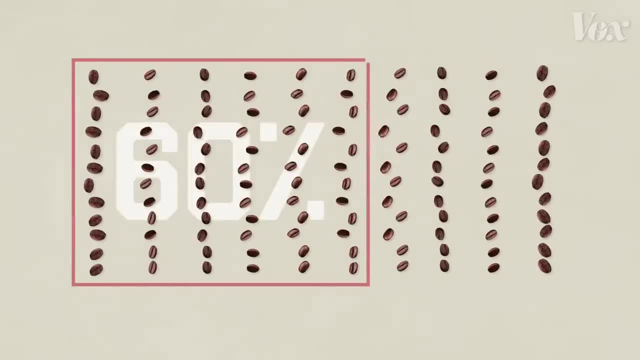 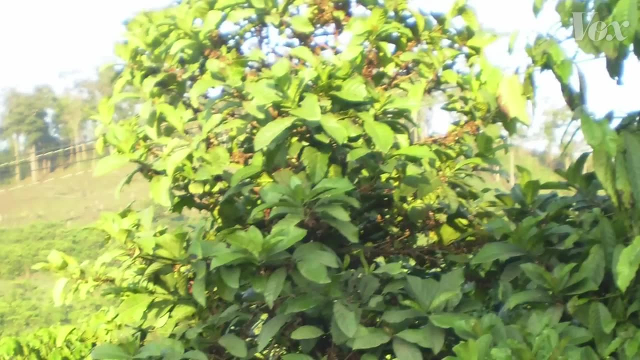 And it's not just cultivated coffee. Another study estimates that 60 percent of wild coffee species could be at the risk of extinction because of climate change. Some of these are used to breed more resistant varieties of Arabica, which makes them critical to sustaining coffee production. 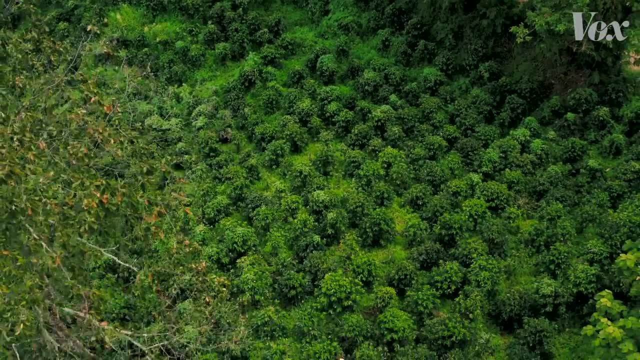 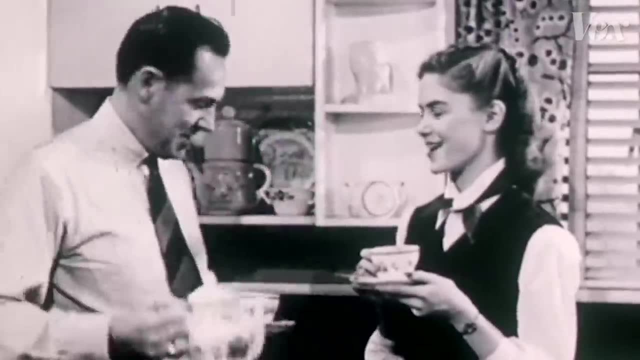 That's not only bad news for the plant, but also for those who have relied on the coffee industry for generations. In the early 20th century, Americans and Europeans were buying more and more coffee. We Americans know what we like, and we really do like coffee. 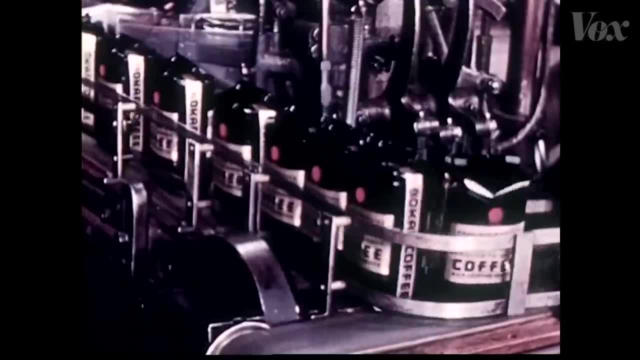 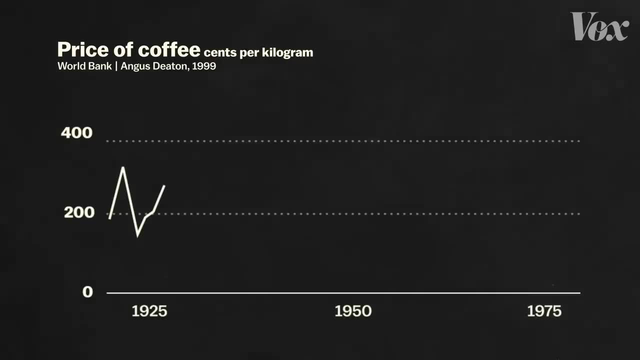 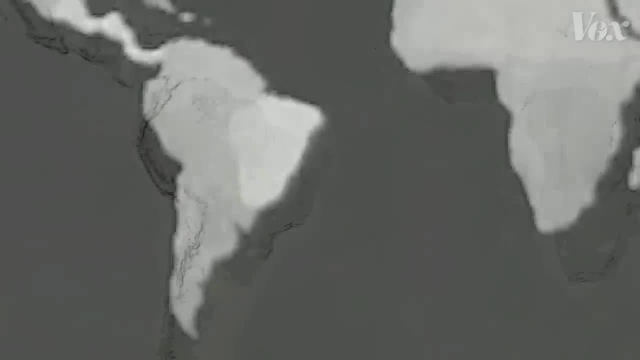 Did I say like? Well, we use more than 3 billion pounds of coffee every year, So prices were high and that created a boom in coffee-producing countries. Where does it all come from? Mostly from South America. So let's fly down and get the story firsthand. 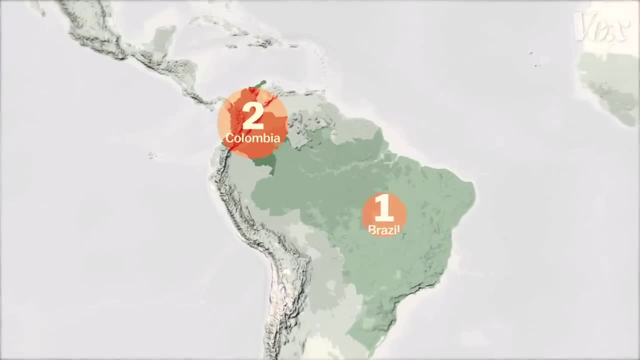 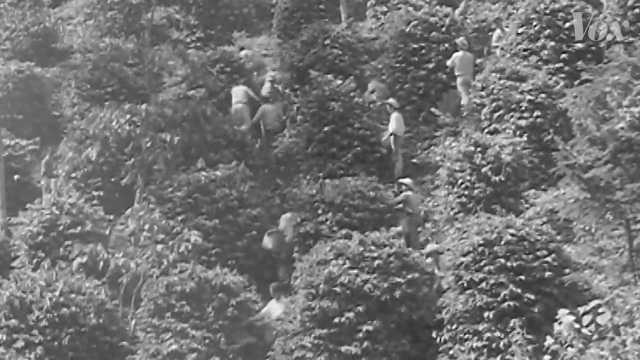 Colombia was the second biggest producer in the world. at the time, It was mostly grown on large coffee plantations called haciendas that dated back to when Colombia was a Spanish colony. The work was done by peasants, indigenous people and former slaves, many of whom were forced off their lands and subjected to brutal conditions. 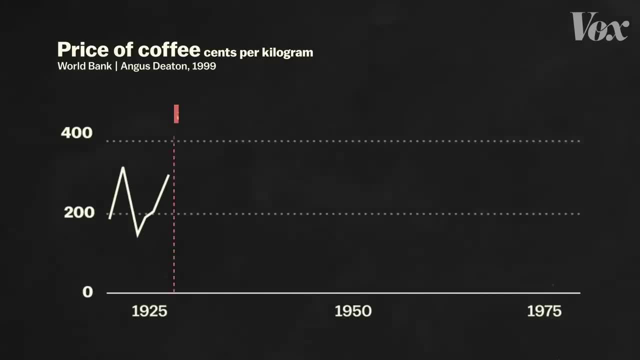 The plantations were profitable while prices were high, but in 1929, the US economy crashed, Demand for coffee fell and so did the price, bankrupting the plantations, Fearing that Colombia's entire coffee industry would vanish. 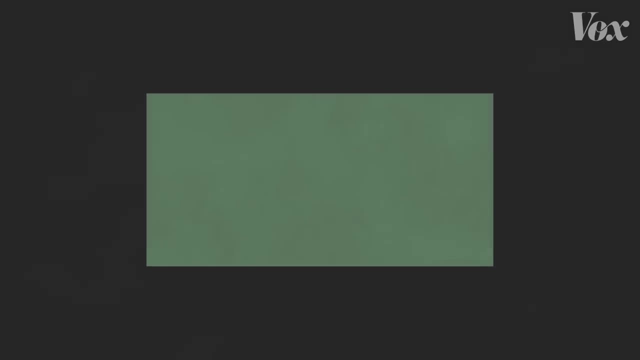 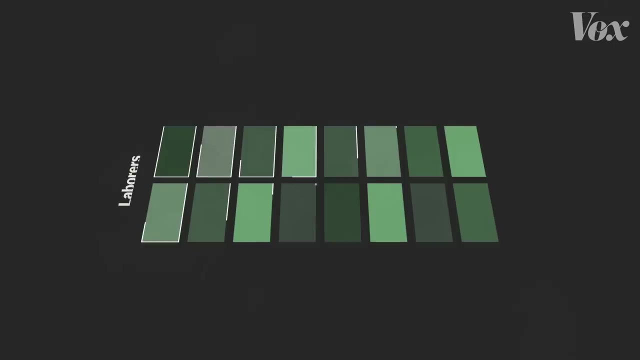 the government stepped in. They purchased these large coffee fields from the owners- Many had more than 1,000 hectares, about the size of 1,800 football fields- And they broke them up into small plots of about 16 hectares each before selling them to laborers. 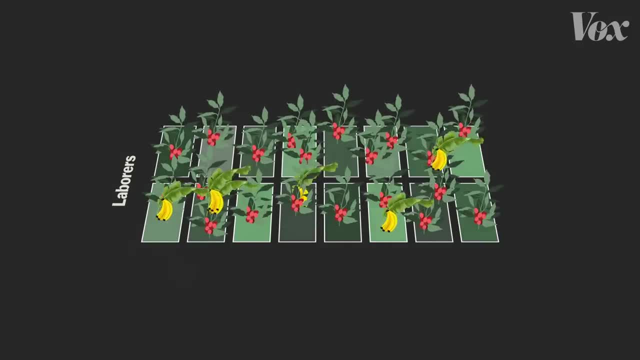 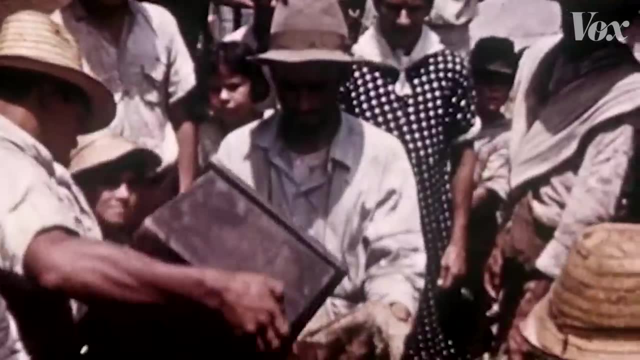 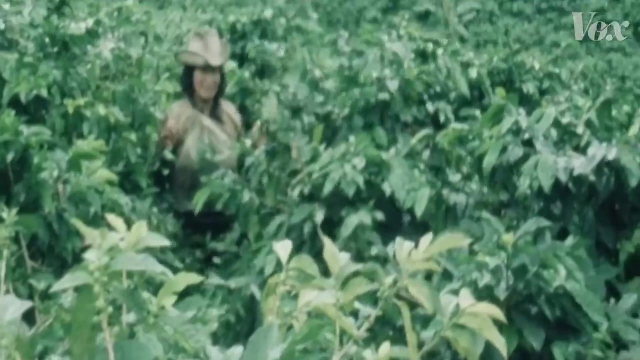 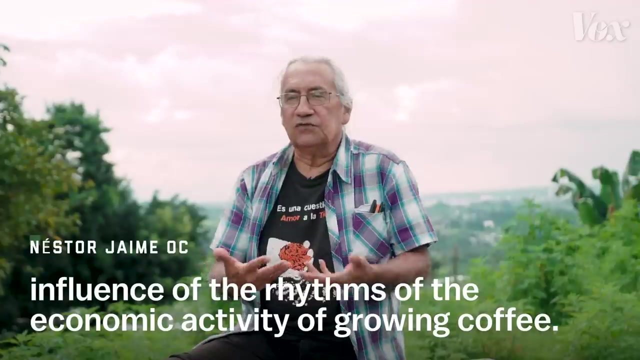 The idea was that these small farms could grow other crops alongside coffee to sustain themselves through price fluctuations. This not only saved one of Colombia's most important industries, but turned it into one dominated by smallholder farmers To support the industry in 1927,. 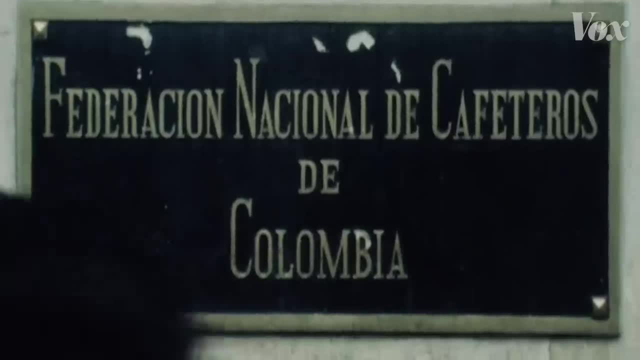 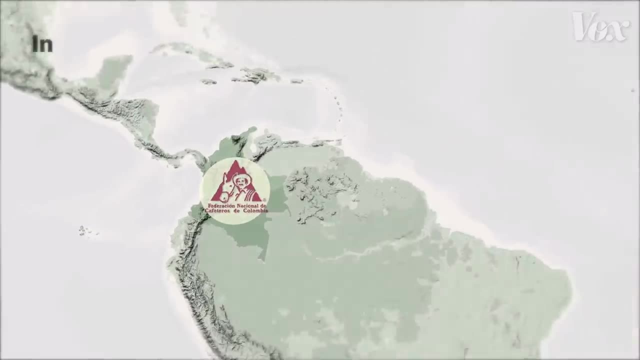 the government had created Fedecafe, an agency that would organize and represent the farmers by negotiating fair prices and favorable deals with other countries. The most important one was in 1962, when Colombia signed the International Coffee Agreement with 69 other countries and set a price minimum for export. 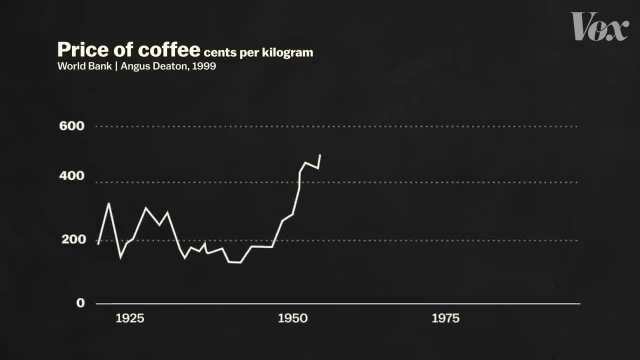 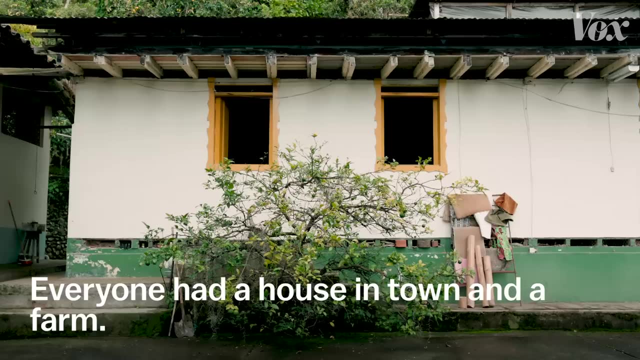 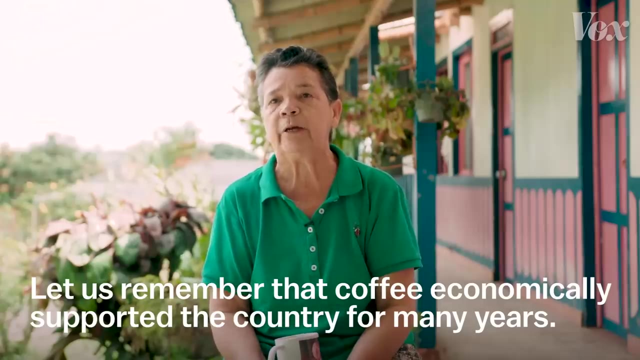 As coffee prices recovered, Colombia's smallholder coffee farmers started thriving. Everyone here had a house in the town and a farm, And we all had to do with coffee. Let's remember that coffee farming sustained the country economically for many years. Let's remember that coffee farming had aces. 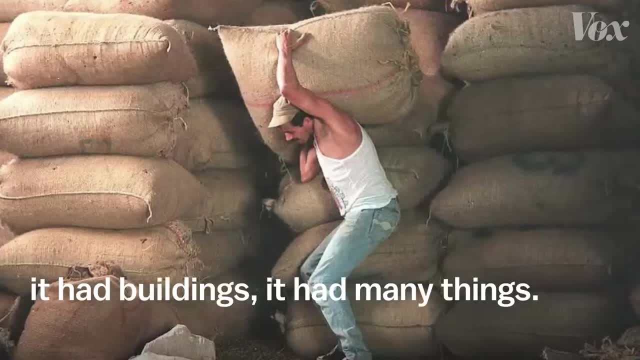 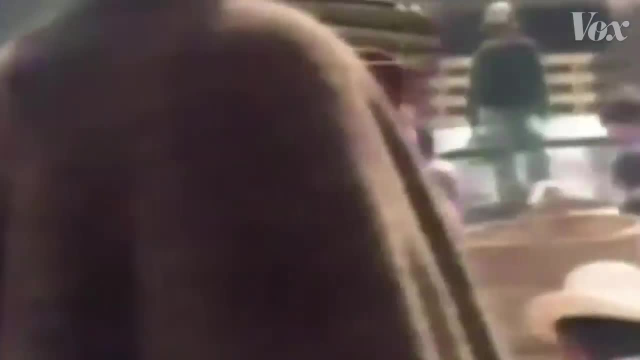 had a Colombian merchant fleet, had buildings, had many things. We were the richest in the country and in the world because we managed a very good price. By the 1970s, Colombia was using the coffee farmer, or cafetero, as a marketing tool around the world. 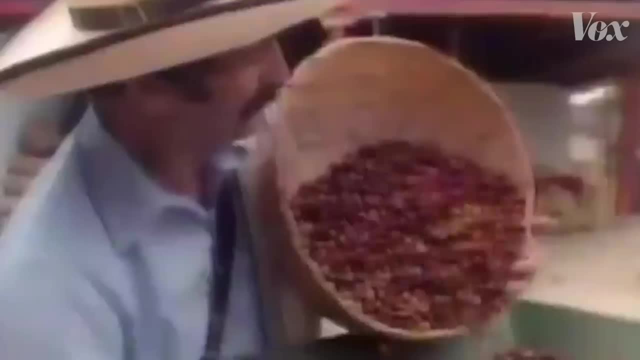 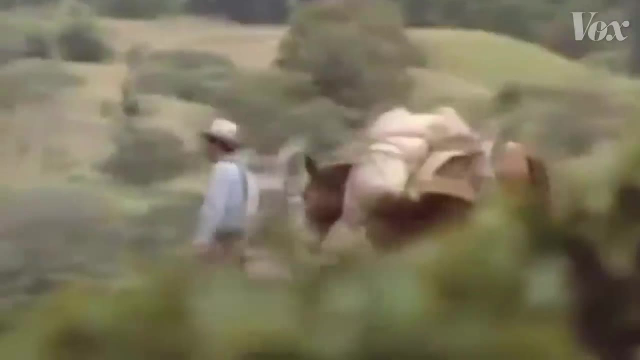 It is here that they buy their coffee, Coffee grown by men like Juan Valdez- Because, for Colombians, their coffee is more than just the richest coffee in the world: It is a national heritage. Today, Colombia is the world's third largest coffee exporter. 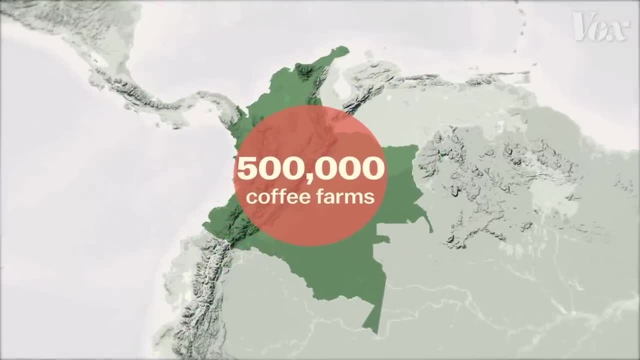 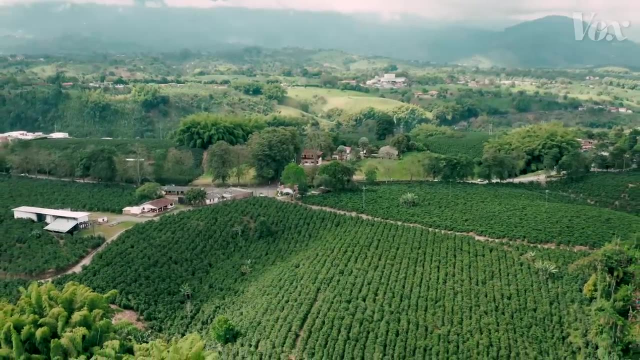 and there are about 500,000 mostly small farms that make up the industry. But just as these farmers are starting to face climate change, the economics that support them are disappearing. There are several ways farmers can protect their coffee plants from the effects of climate change. 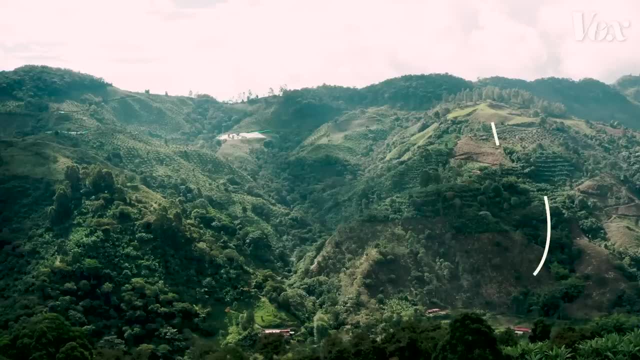 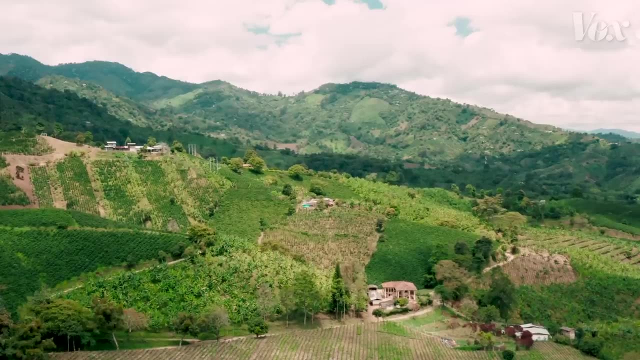 Shade trees keep the plants cool and stabilize the soil. Farmers can move their crop uphill where it's cooler. They can also switch to more resistant varieties of coffee plants. The problem is, all these solutions cost money that many smallholder farmers don't have anymore. 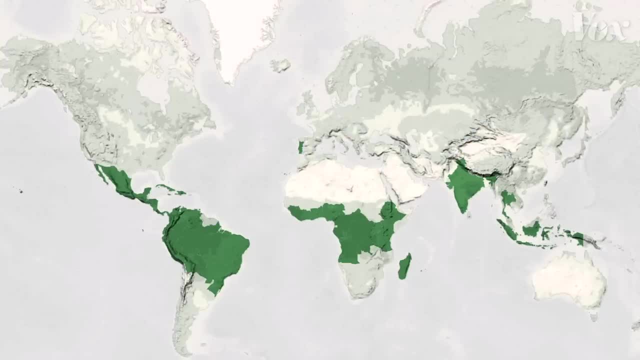 It started in the 1980s, when the coffee agreement fell apart along with the price minimum. Since then, more countries, especially some in Asia, have increasingly flooded the market with cheap coffee. It sparked a crisis around 2009,, when extreme weather and coffee rust. 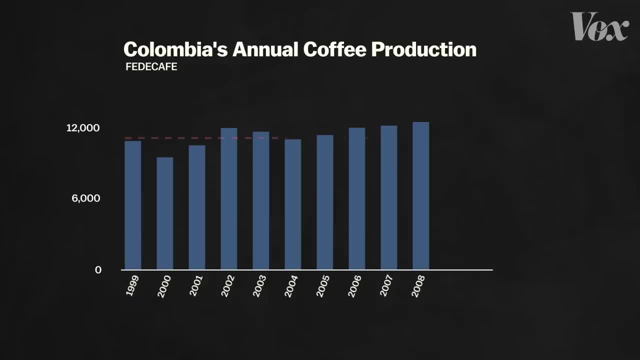 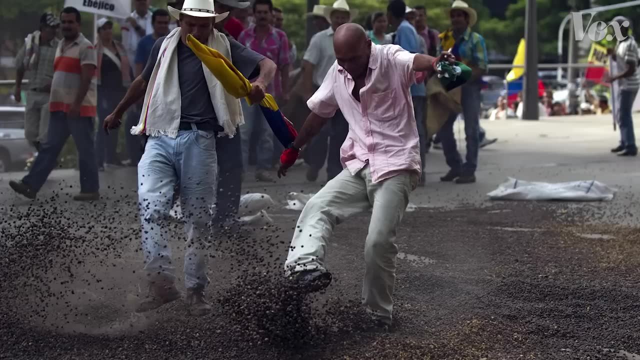 decimated. Colombia's crop Production fell to its lowest levels in decades In 2013,. thousands of farmers went on strike and demanded that the government provide them with more financial support and establish a reasonable price minimum. The government increased subsidies to coffee growers. 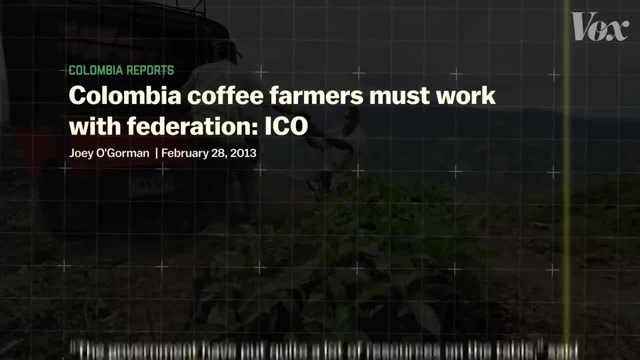 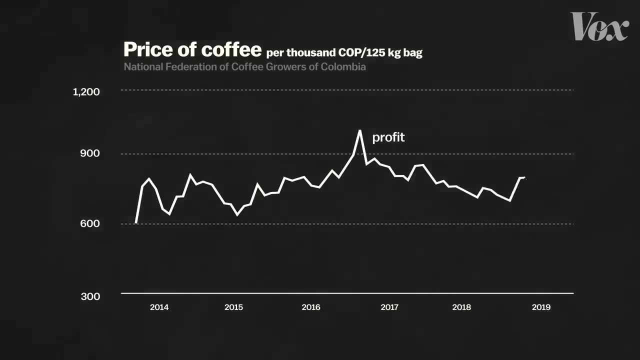 but without another international coffee agreement, a return to a price minimum was no longer possible, So coffee prices continued to fluctuate. Today it's below what many farmers need to break even. That's why it's so hard for these farmers to adapt to climate change. 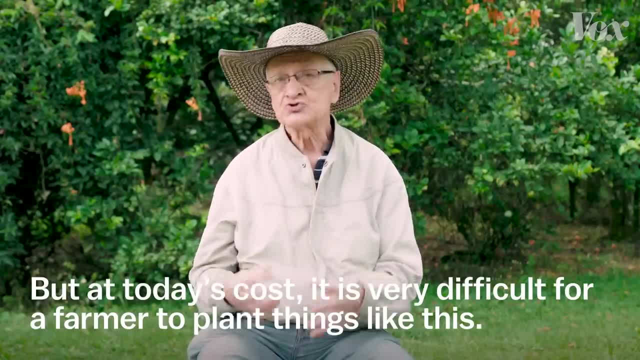 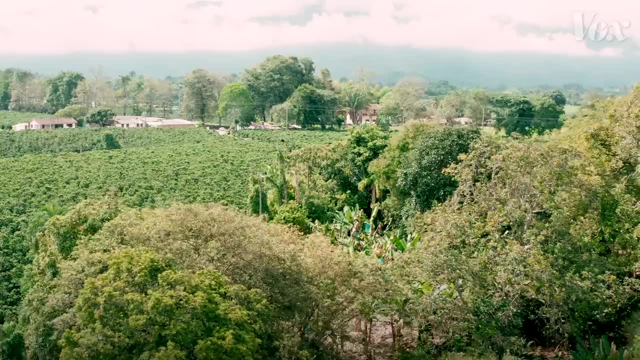 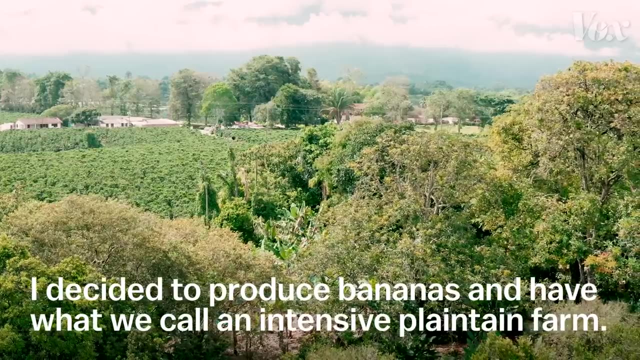 But today, at today's cost, it's very difficult for a farmer to grow coffee like this. It's forced many farmers in the Zona Cafetera to replace coffee with other crops. I started growing bananas in what we call here an intensive banana cultivation. 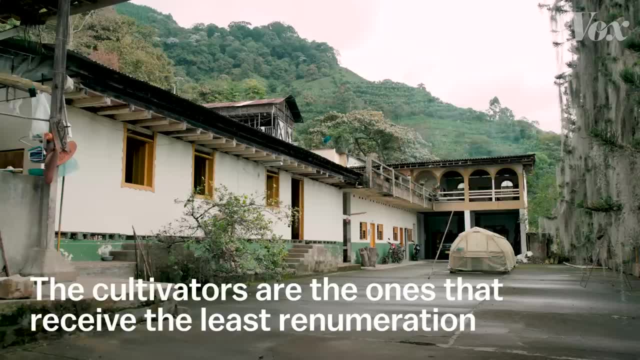 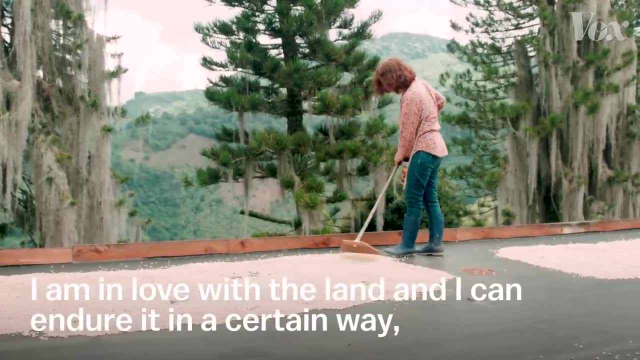 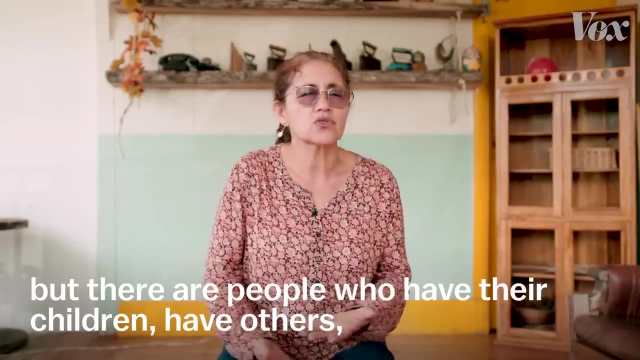 So the growers are the ones who receive the lowest pay. So people get tired. I mean, I'm in love with the land and I can handle it somehow right, But there are people who have their children, who have other. I mean they have a lot of responsibilities.